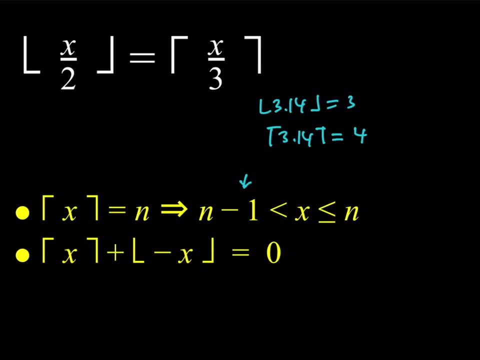 again as an example, if you take the opposite of the 3.14, that's going to be negative 3.14, and then its floor value is going to be negative 4, as you know, because you're supposed to be rounding it down right and in this case you're talking about the. 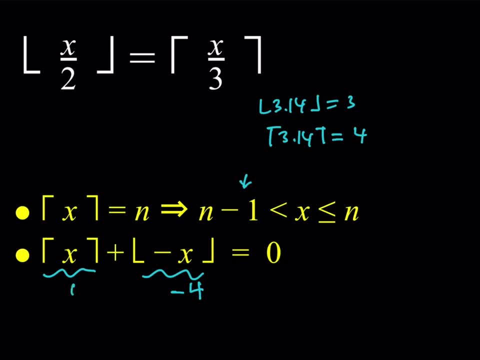 ceiling value of 3.14, which is 4, and their sum is always 0.. Okay, so, given those, let's go ahead and take a look at this problem. So we do have. the floor of x over 2 is equal to the ceiling of x. 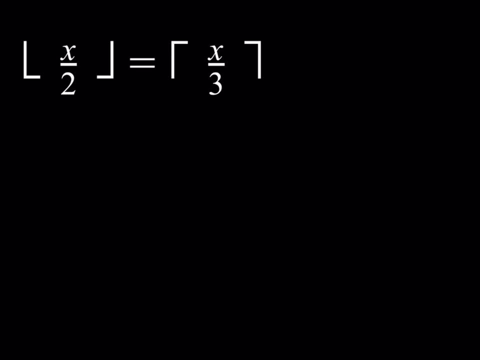 over 3.. So, as almost all the time, we're going to set this equal to an integer, n. so in this case we know that n is an integer and we're going to try to solve for possible values of n. Of course, this is not going to be x, but we also need to know our boundaries for n. Okay, so using the first, 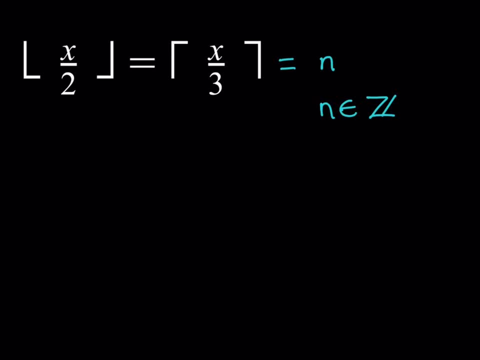 part, which is the the floor function. let's go ahead and write down what we have. So, since the floor of x over 2 is equal to n, this implies that x over 2 is between n and n plus 1.. Now remember that on on the lower side, we always have the equality and the lower number is always n, with 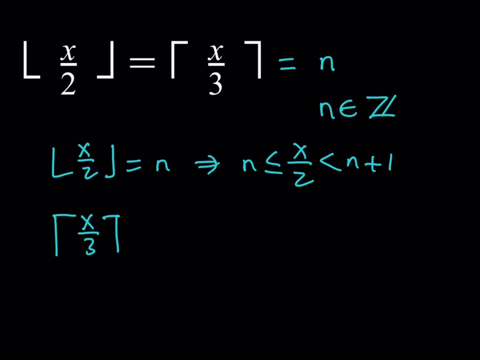 the floor function. On the other side, with the ceiling, it's a little different. Things are a little different. Things are a little different. little different because what you're supposed to do is you have to put the n minus 1 here with no equality, and you have to put the n on the other side, with the equality, because, remember that, 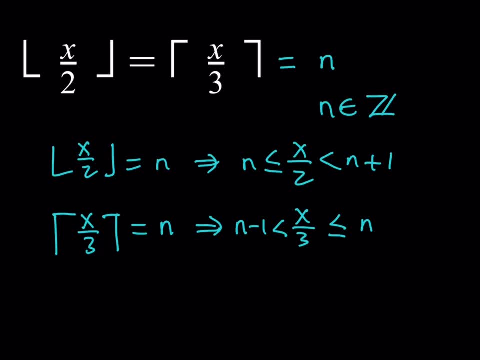 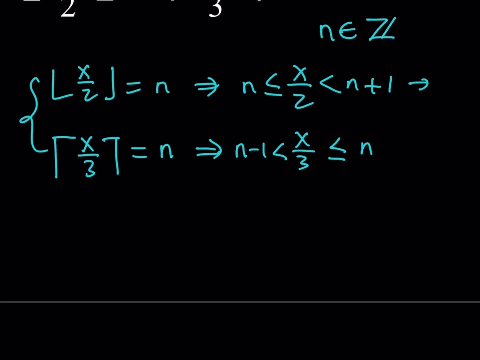 if a number is an integer, then its floor value or the ceiling value is always going to be the same number. Okay, so now how do you put these two together? Well, I'm just going to go ahead, and, you know, isolate x in these inequalities. so let's go ahead and multiply both sides. or I should say: 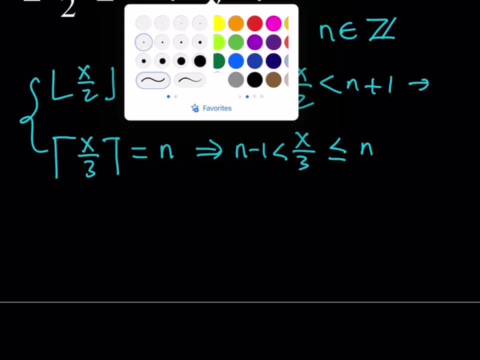 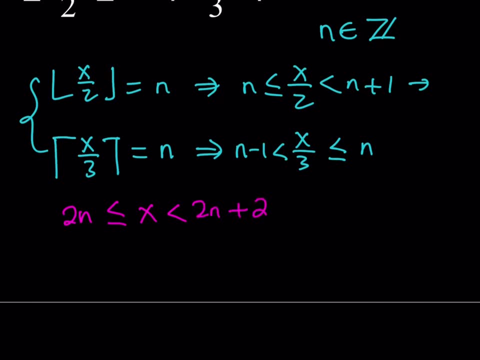 everything by 2, so that should give me something like 2n- x and 2n plus 2. and the second inequality: if I multiply everything by 3, you get 3n minus 3, with an x in the middle and 3n on the. 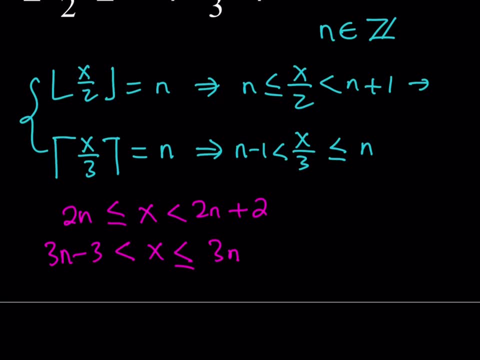 right hand side. Okay, great, so we kind of have like two double inequalities and we're going to solve these. but remember that n is always an integer and one of the strategies that we use for these kinds of addition, so and so and chain of inequalities is that we take the lower value from one of the inequalities and we take 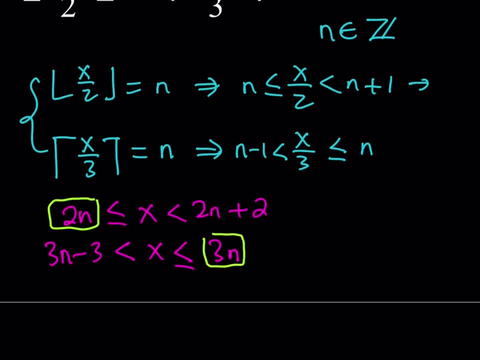 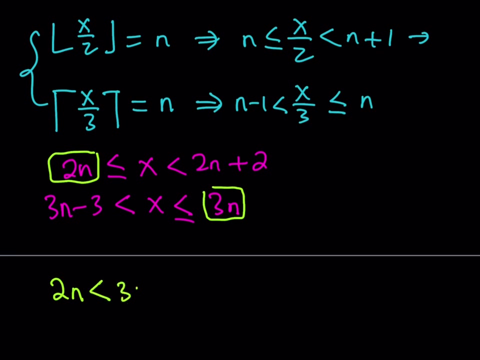 the higher value from the other one and we compare them. Obviously, x needs to be greater or equal to this and less than that. therefore, the upper limit or upper boundary needs to be greater than the lower boundary in this case. Okay, so we can safely say that 2n needs to be less than 3n. Okay, and 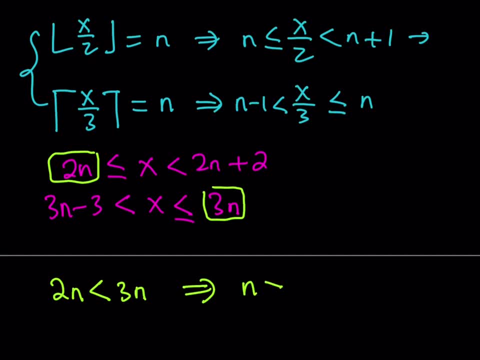 this implies that n is greater than zero. If you go ahead and isolate n on one side, you're going to get that n is equal to, I mean n is greater than zero. This shows that n has to be positive, which also means that x needs to be positive. right, obviously. How about the second one For the 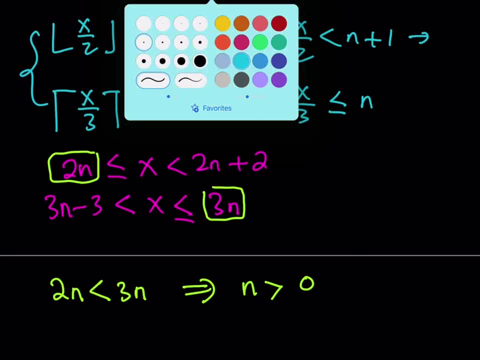 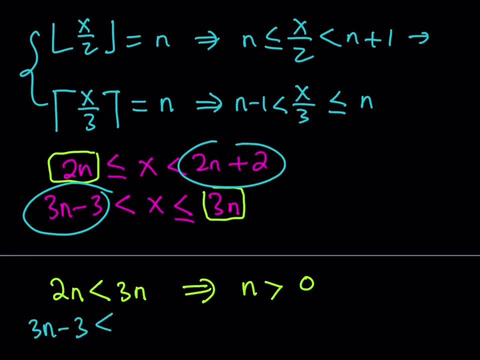 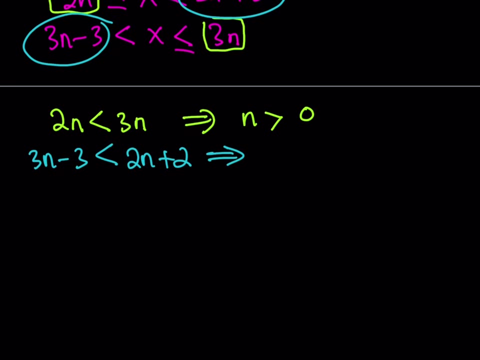 second part. we're going to be doing something similar, obviously right. We're going to be comparing this one and this one, and this tells us that 3n minus 3 needs to be less than 2n plus 2. and what does that imply? If you subtract 2n from both sides, that's going to give you n is. 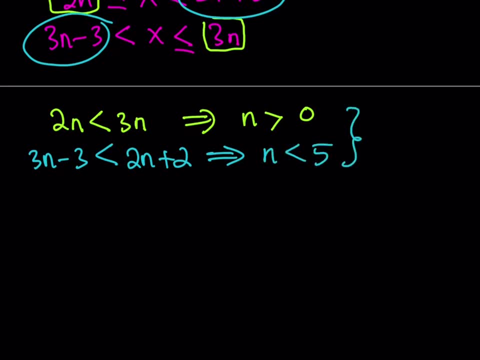 less than 2n. So if you subtract 2n from both sides, that's going to give you n is less than 2n- Great, so remember that both of these have to be true. so we're going to look at the intersection. and also, n is an integer. What is that supposed to mean? This means that n is between zero and five. 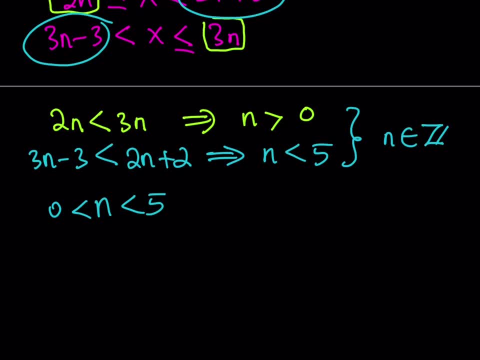 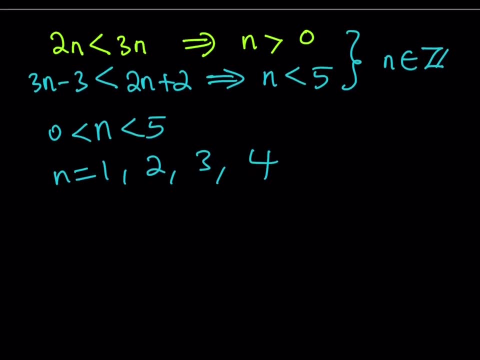 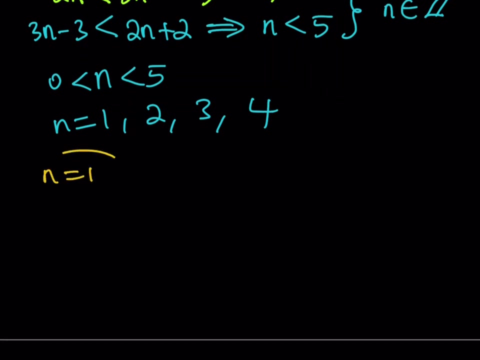 okay, and that's not inclusive. n is an integer, so n can be one, two, three or four. Let's take a look at each case, because each case is going to give us interesting results, and let's go ahead and explore what happens. So I'm going to be looking at each case separately and we have to be very 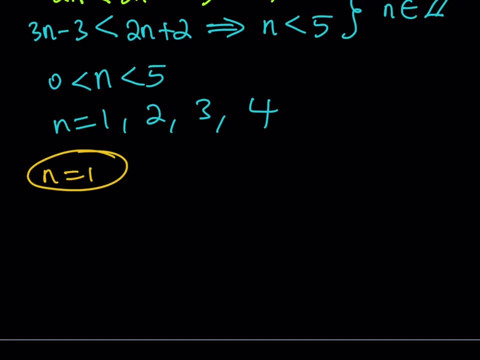 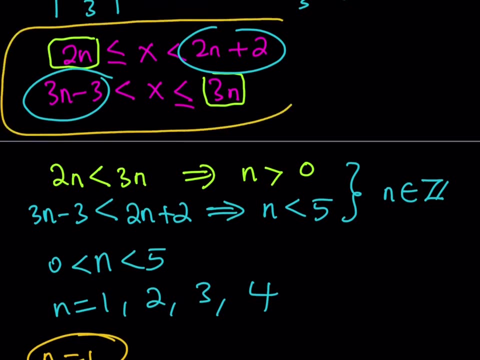 careful. Now, if n is equal to one, what happens, right? Okay? so if n is equal to one, I'm going to go ahead and substitute my value for n here and here. then I'm going to look at the intersection of those two inequalities. So that's pretty much what I'm going to be doing all the time. okay? So if n is, 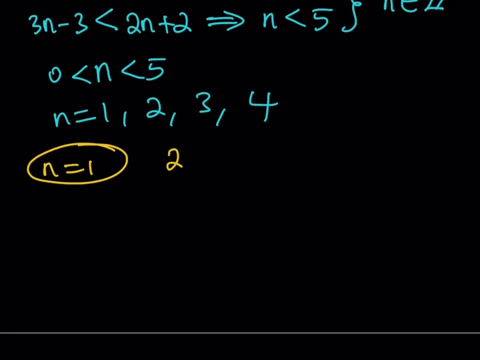 equal to one, then I should be getting something like: well, x is between two and four and between zero and three. Okay, if you look at the intersection of these two inequalities, you're going to notice that it has to be between two and three inclusive. So that's what we're going to get from the first. 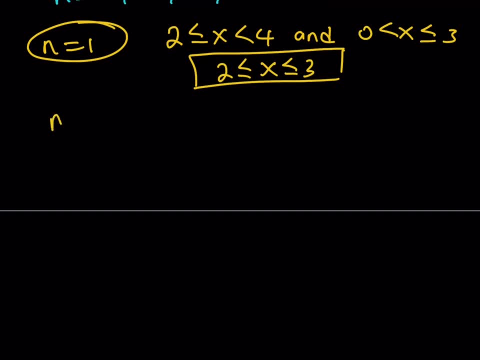 value of n, which is n equals one. Okay, let's take a look at n equals two. If n is equal to two and you substitute that into the inequalities that we have, we're going to be getting something like this: four and six here and three and six here. Notice that these two numbers are always three apart, and 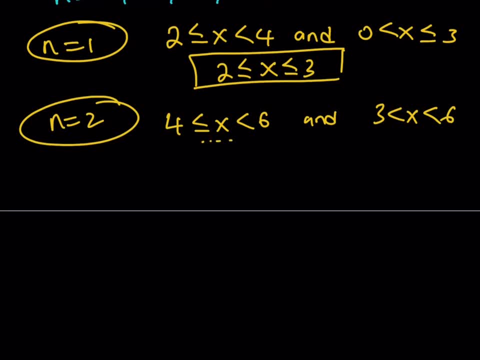 these two numbers are always two apart. These are two apart and these are three apart. That's basically going to repeat over and over And obviously, if you look at the intersection, you're going to notice that x needs to be between four and six, but it can also equal four, but not equal. 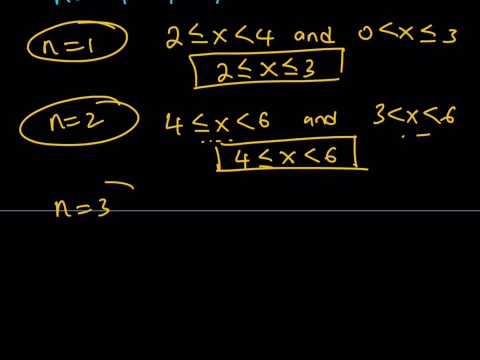 six, Okay, and then we're going to be looking at: n equals three. If n is equal to three, then x needs to be between six and eight, and six and nine, All right. this means that x needs to be between six and eight, but not inclusive. All right. and finally we're going to 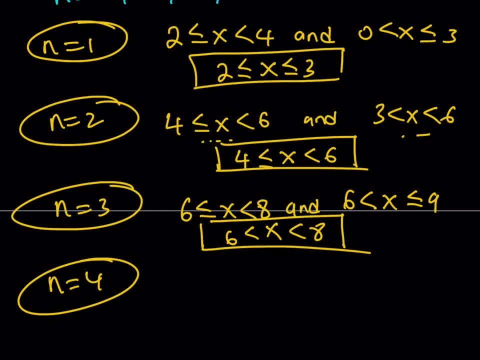 be looking at. n equals four. Let's see what that gives us. That's going to give us eight and ten here, and on the other one we're going to be getting nine and twelve. Obviously, every time the lower boundary is also increased by three. so that's going to be nine and twelve And the 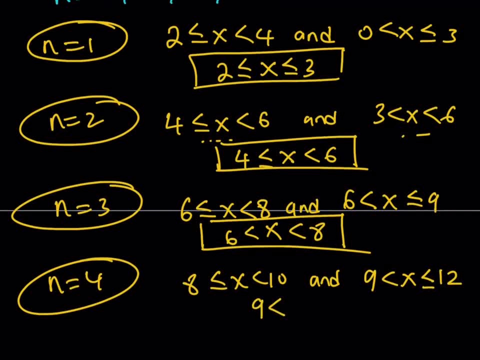 intersection of these two inequalities is going to be between nine and ten. None of them are going to be inclusive. Okay, so we basically got four inequalities. Now notice that x, in this case, can be an integer. sometimes, For example, x equals two is an integer solution. Three is an integer solution. Four is an integer solution. 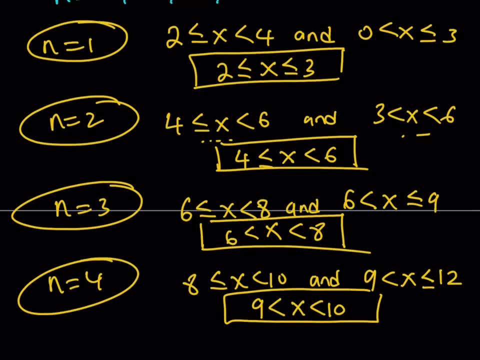 Obviously, five is an integer solution and seven is an integer solution. Those are all the integer solutions And if you go back to the problem, you're going to notice that you can substitute and verify those. But not only that, it's also going to be four of these inequalities. So, but